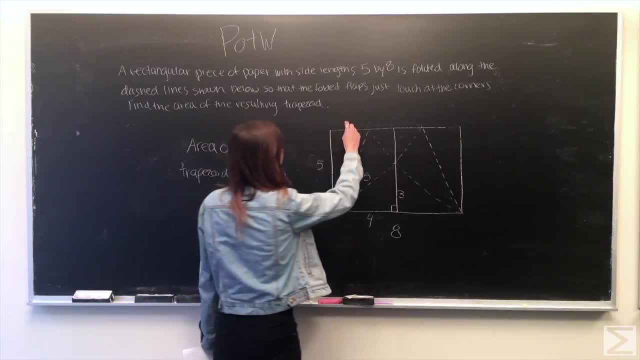 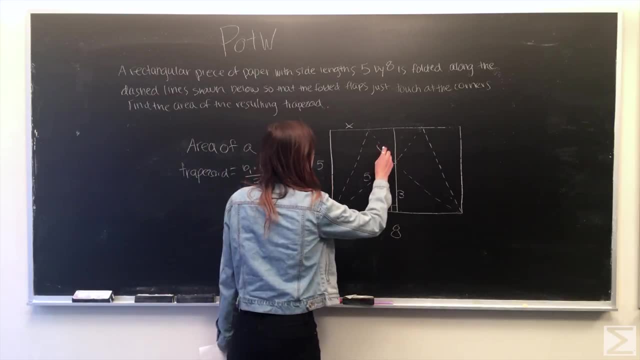 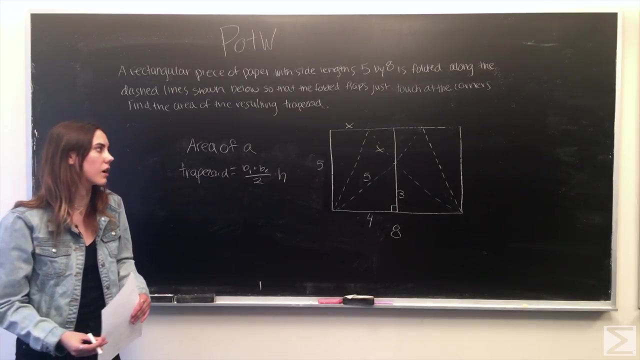 corners of the paper over. if we call this part x, the reflection of x over the folded line is actually also here, and what we can then do is try and solve for the top base of the trapezoid and then plug in what we know from the fold and 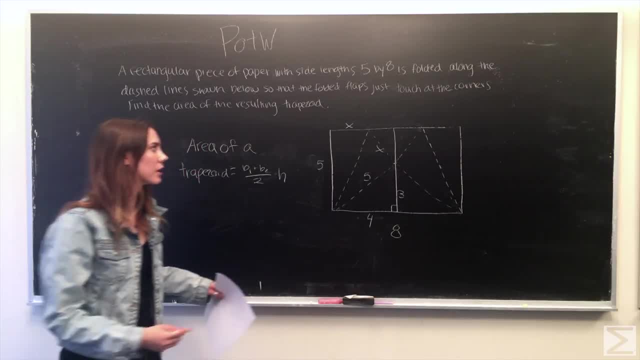 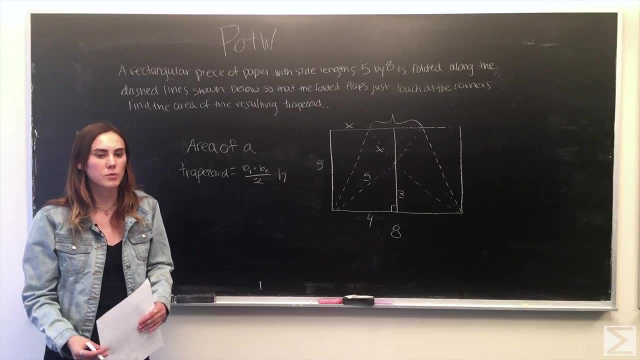 then plug in what we know from the fold and then plug in what we know from the for the area. so we really want to find this area here and what we can do. we can kind of do a similar thing where what we did with the base and we bisect it into. 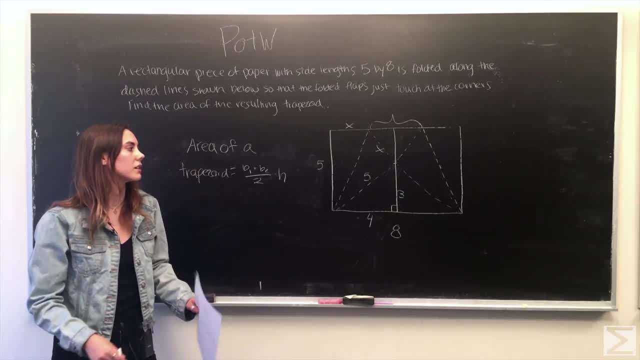 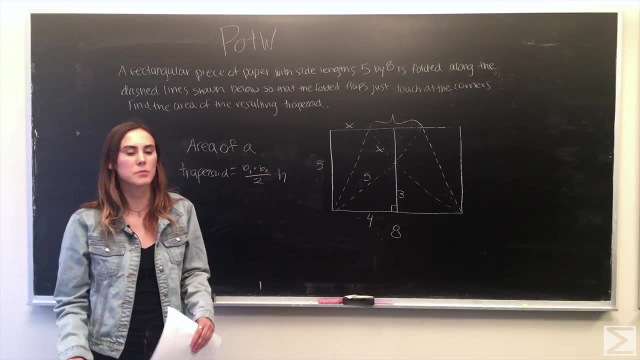 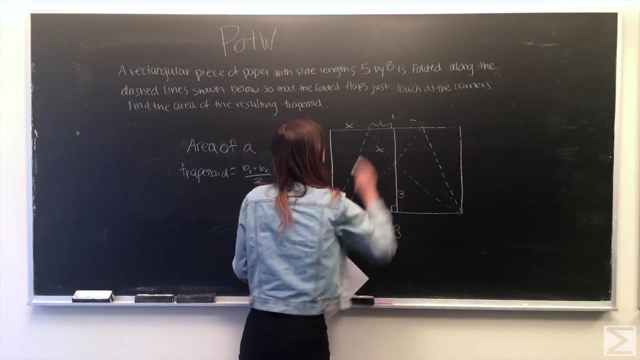 two triangles that make up that area and using the new variables X, we can use the Pythagorean theorem to solve for what the base is equal to. so we know that this area is actually equal to four minus X, just based off of the bisection. 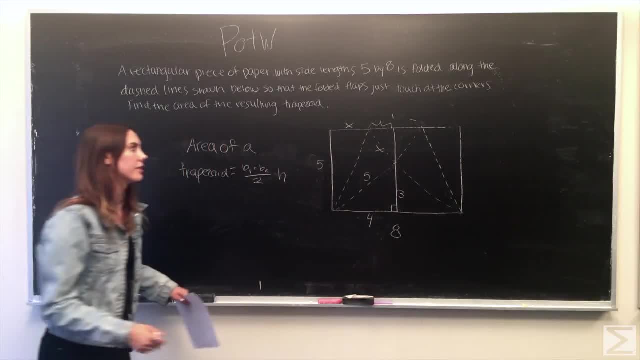 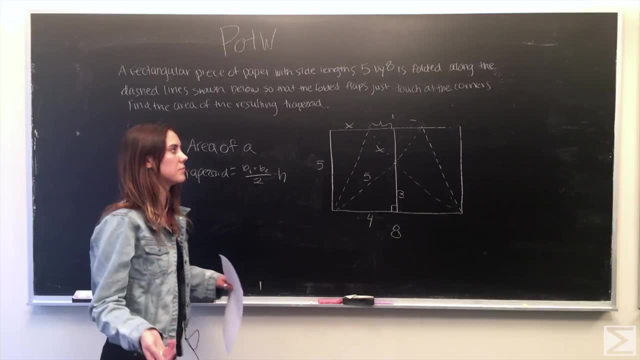 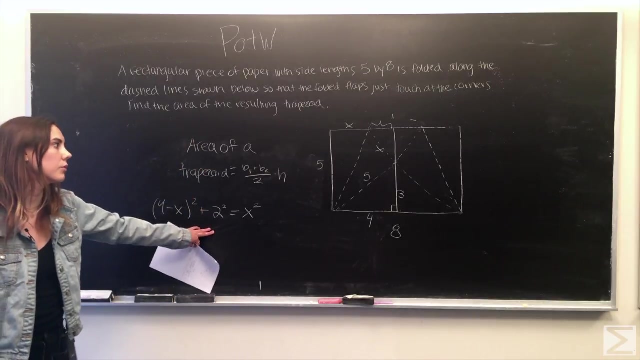 here we know that this is four, and so that half of the base has to be four minus X, and then we can use the Pythagorean theorem to solve for what half of the base is equal to. and we actually get this two from this line here. 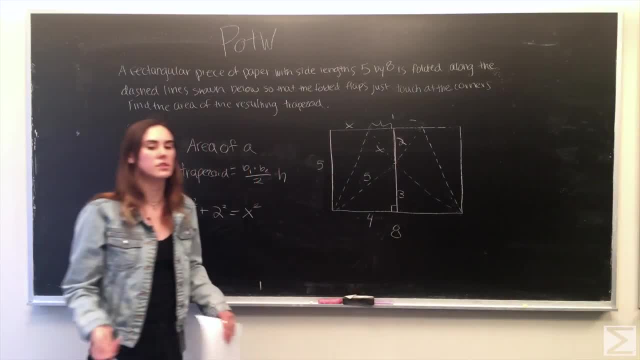 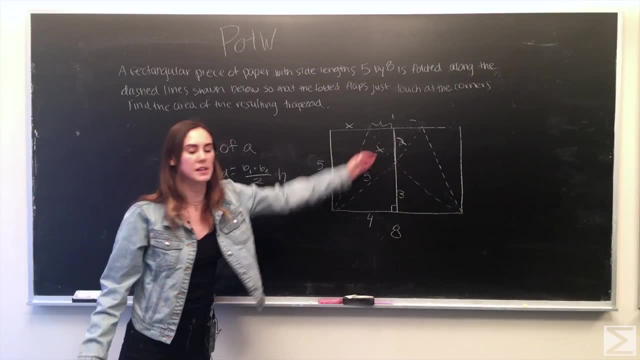 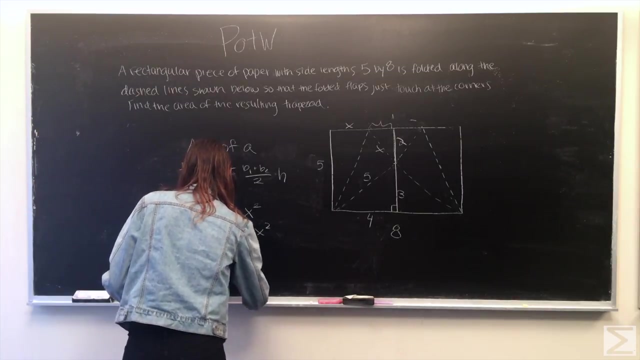 We can just solve for that simply by knowing that the height of the paper is 5, and we know that up until this point, the height is 3, so this has to be 2.. And just doing some algebra to solve this out. 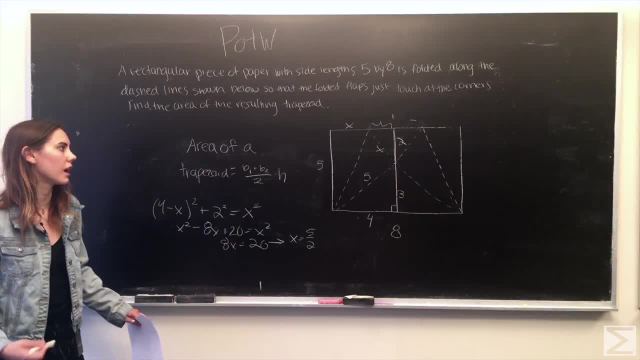 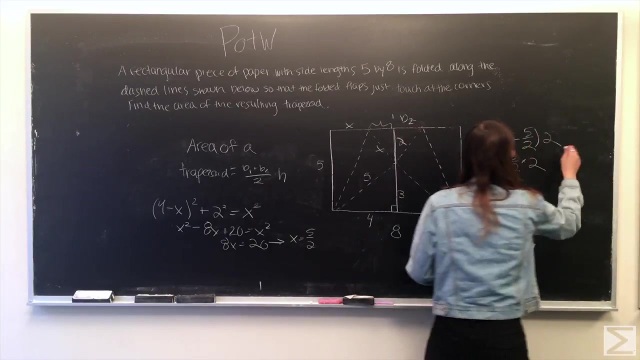 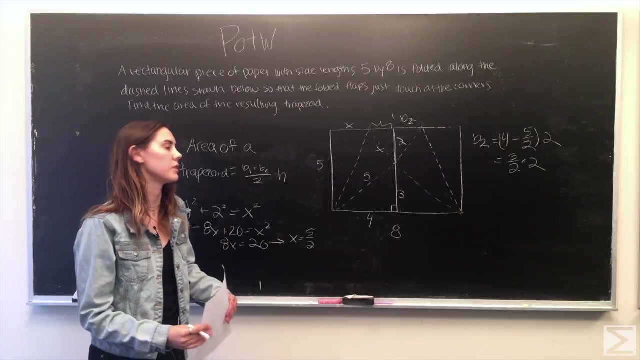 What we get is that x is equal to 5 over 2, and we can solve for half of the top base of the trapezoid by subtracting x from 4.. So then we know that the top base is actually equal to 3 over 2 times 2, because we have 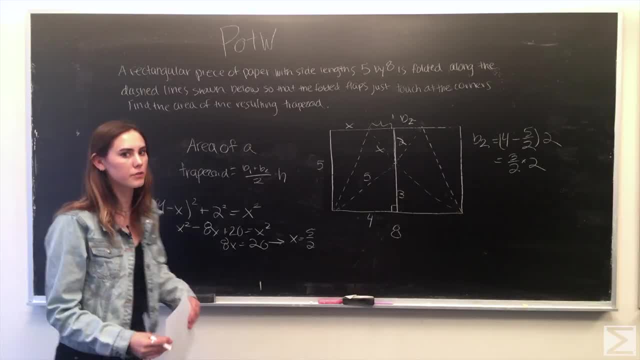 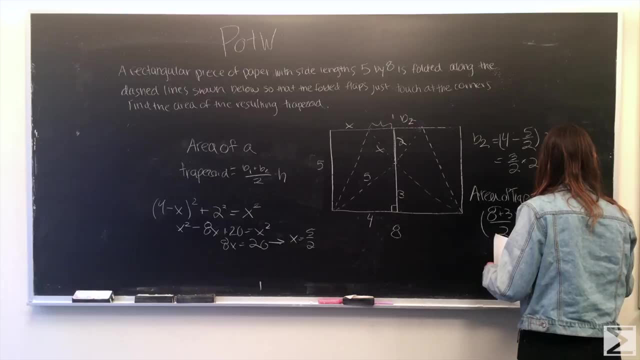 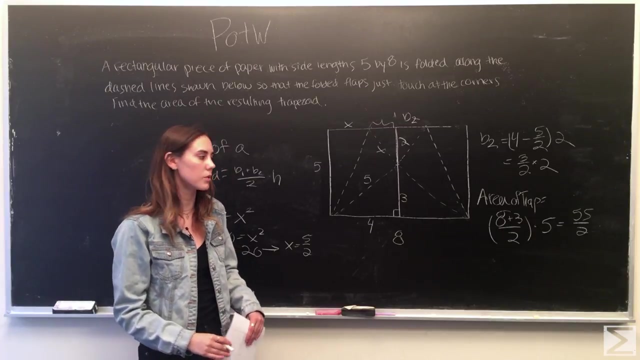 only solved for half of it. Now we just plug everything in and we can solve for the area of the trapezoid. So, plugging in, we get 8 plus 3 over 2 times 5 is equal to 55 over 2, which is 27.5.. 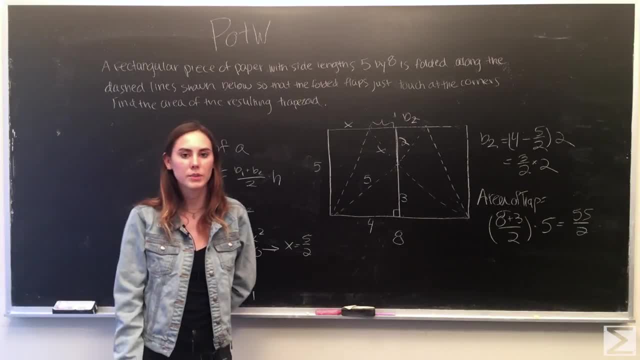 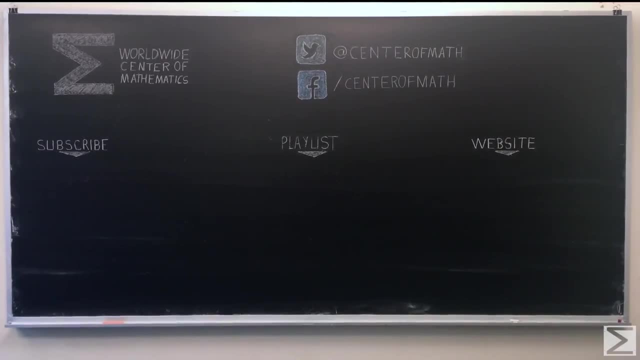 That's all we have for you today. I hope you enjoyed watching this problem. Please check out some more of our videos on YouTube. check us out on Facebook and subscribe on Twitter. Thank you, Thank you.